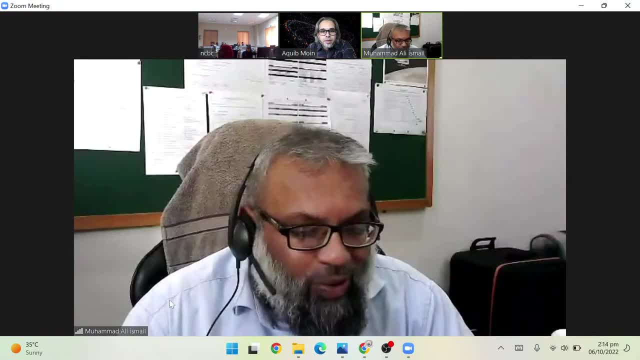 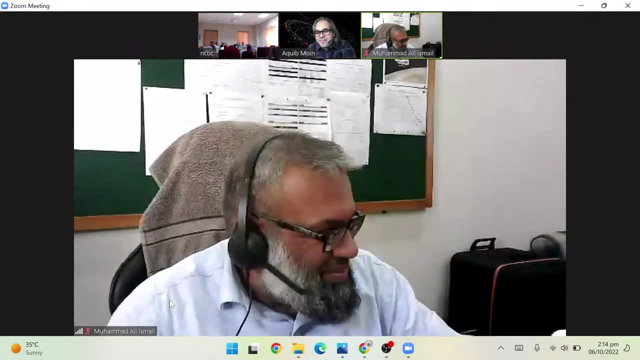 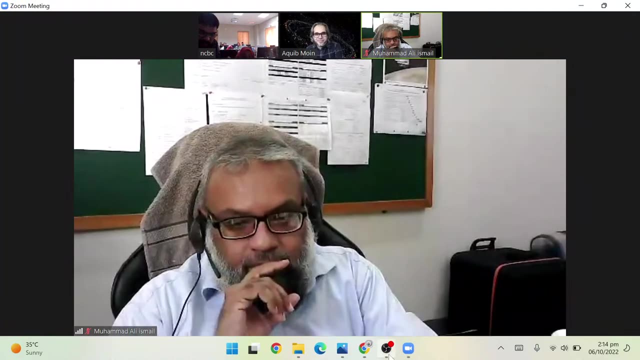 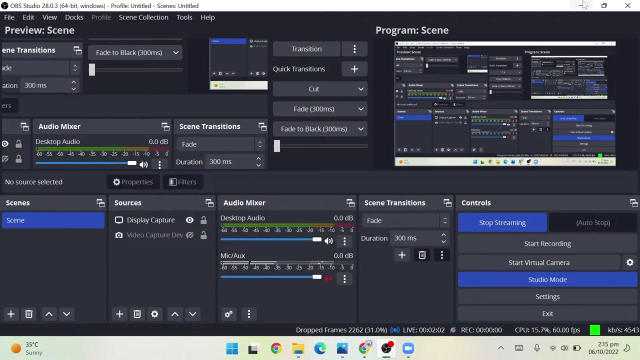 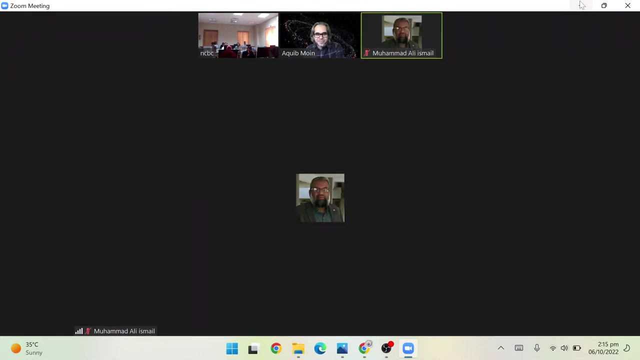 Absolutely. I'm ready. Okay, So I am meeting myself now. Floor over to Hira. Thank you, Hira. Good afternoon. Thank you everyone. Thank you The last people, the last following committee members, thanks all of us. 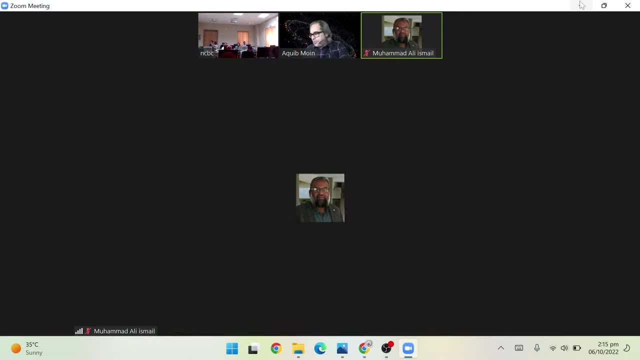 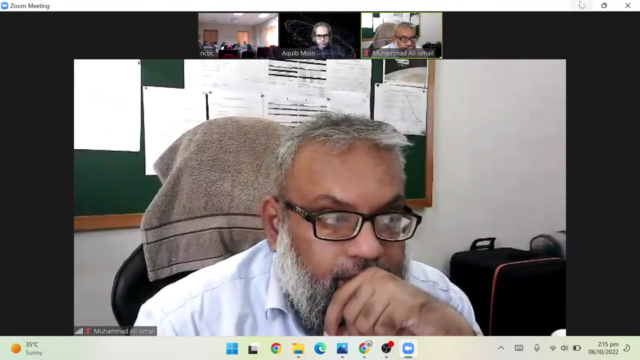 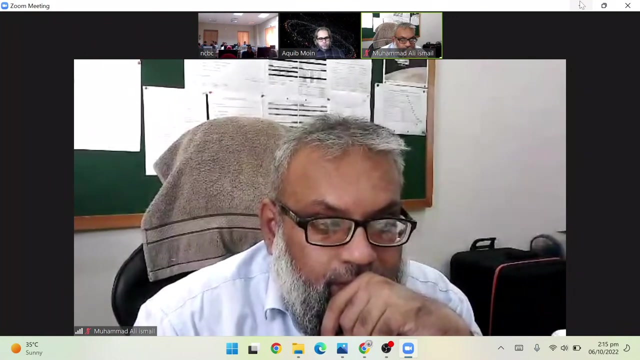 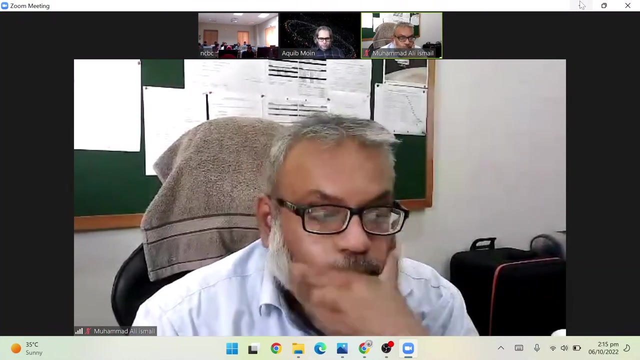 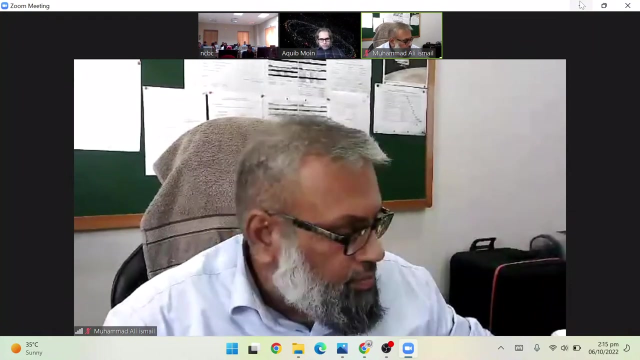 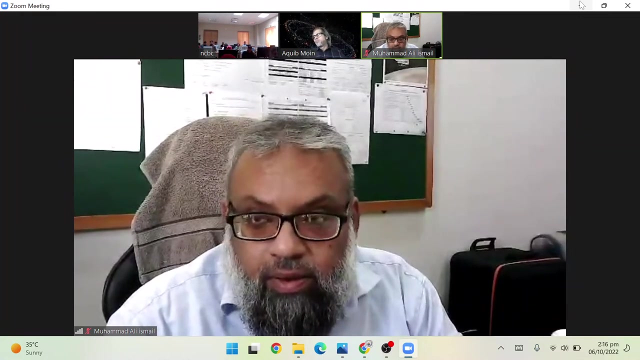 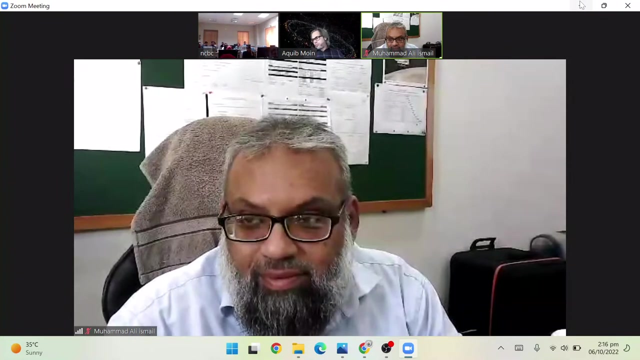 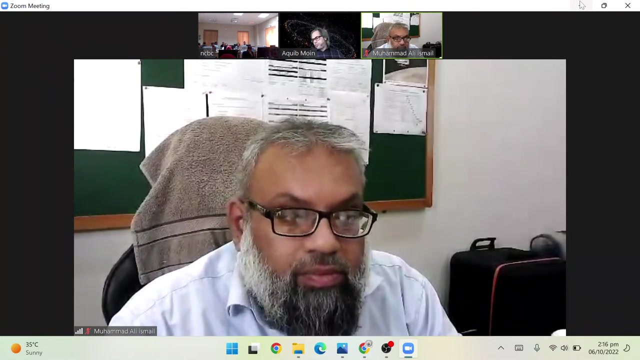 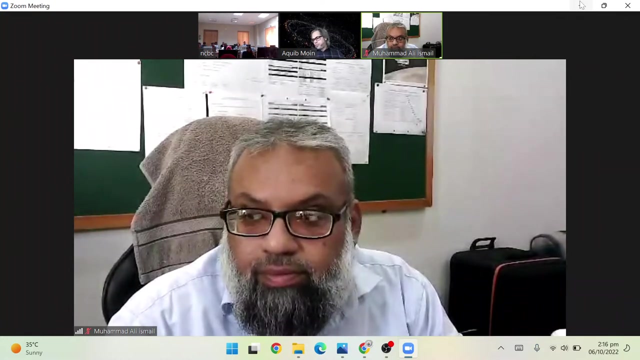 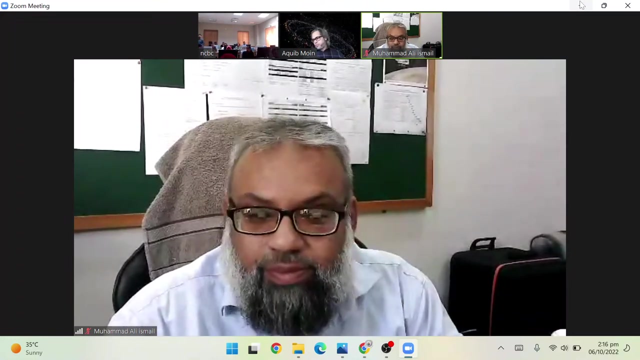 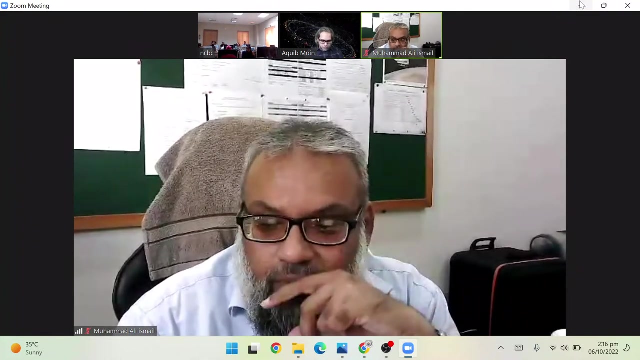 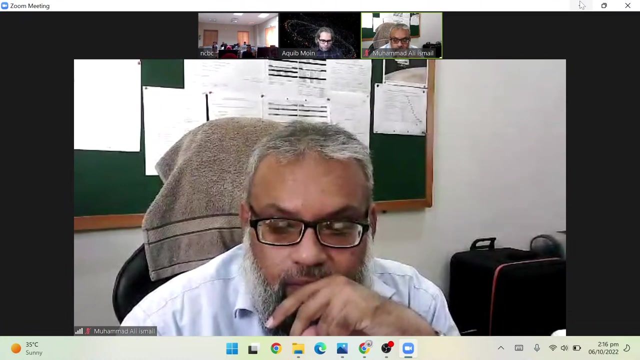 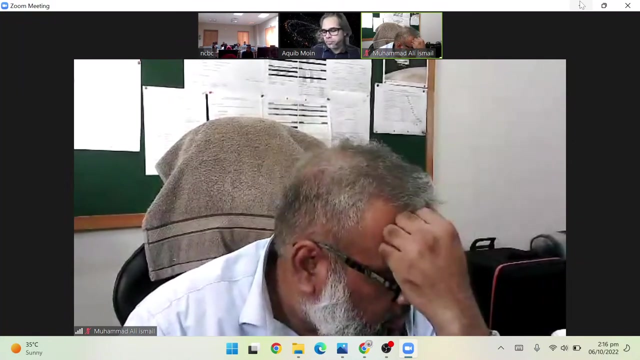 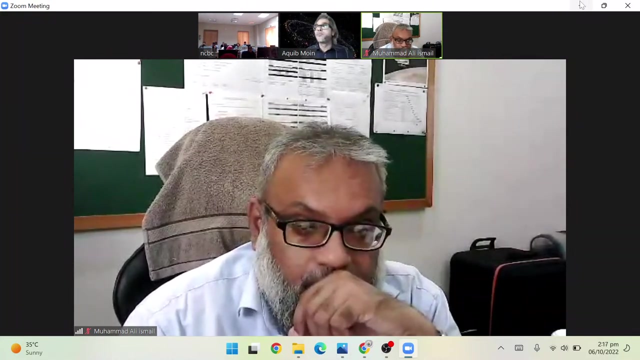 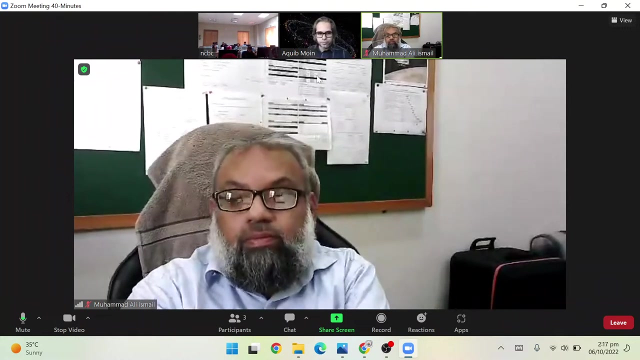 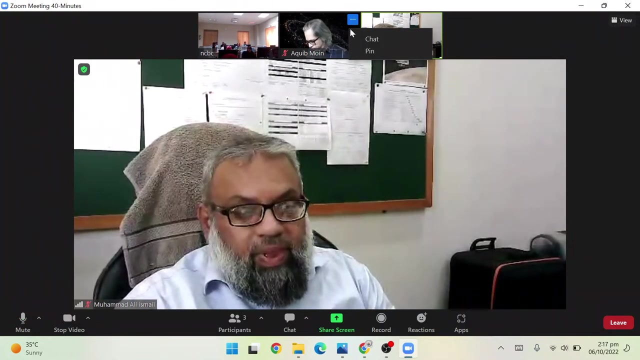 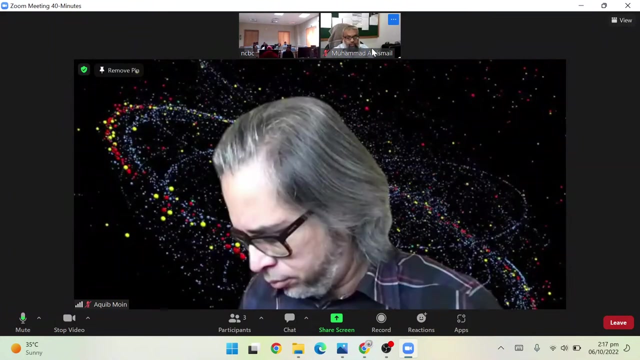 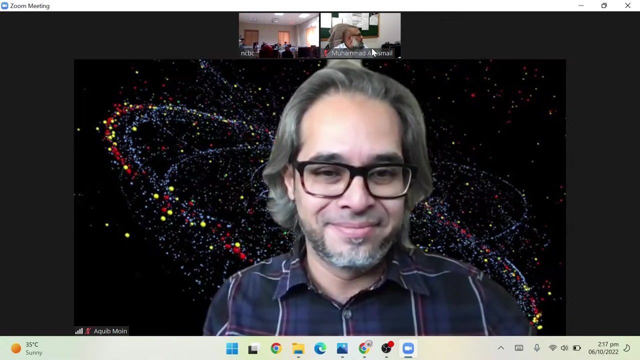 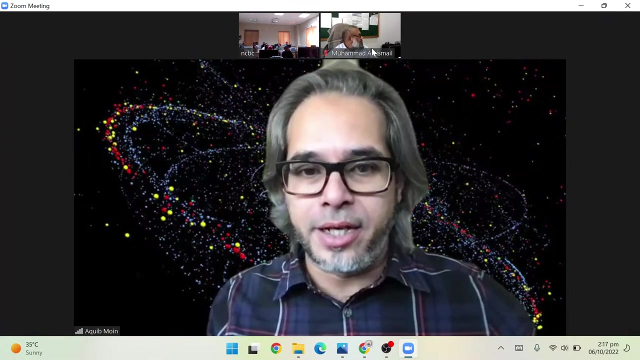 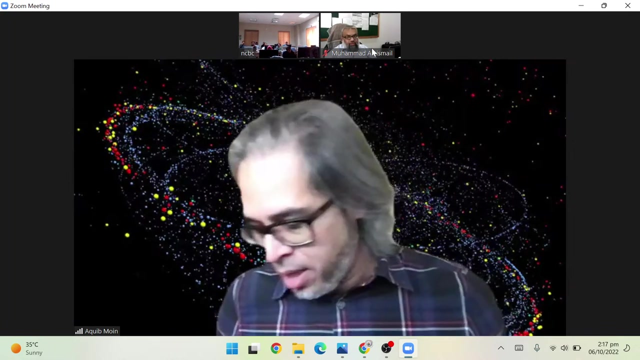 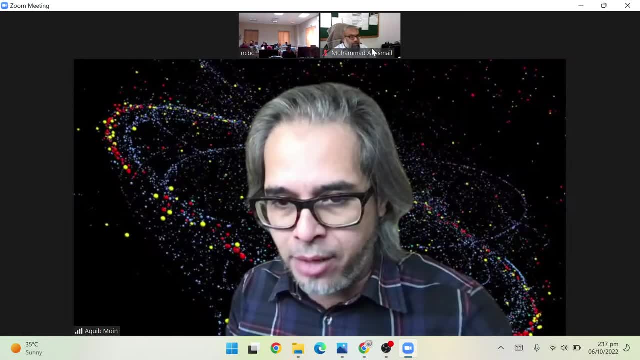 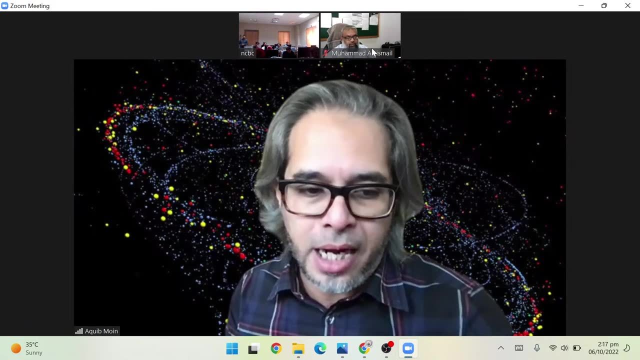 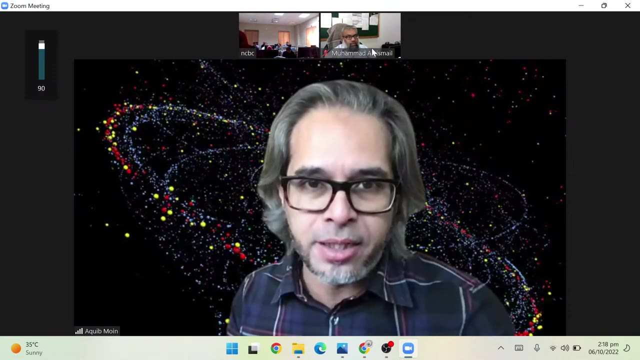 introduction, And I'm really glad to be giving this talk today, And so NCBC and I go a long way. We have interacted before. I visited NCBC as well, So it's a pleasure for me to be a part of the NCBC. 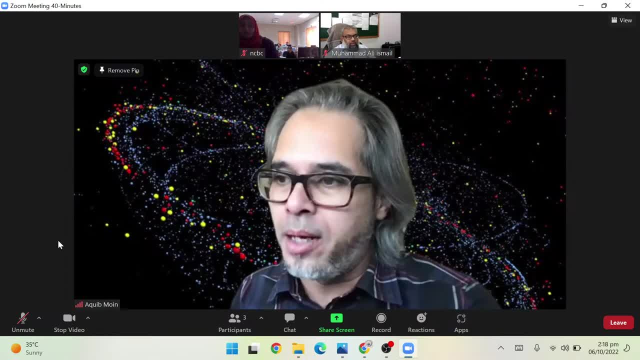 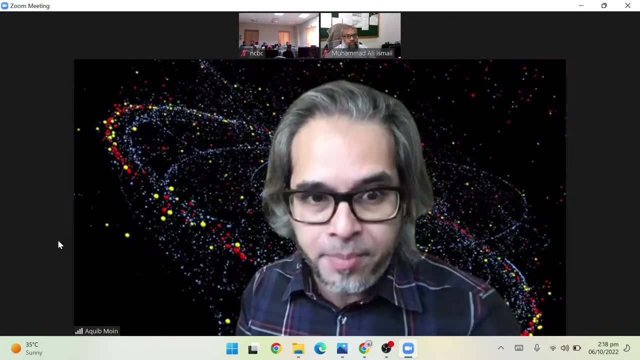 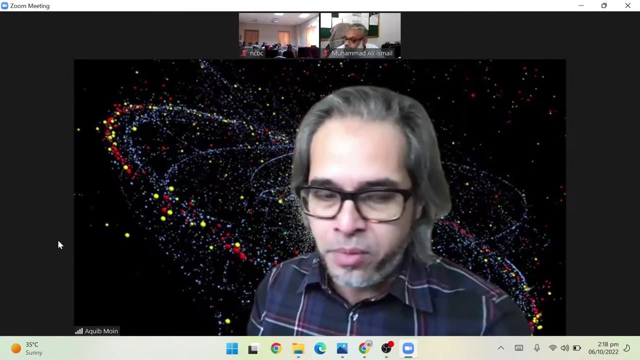 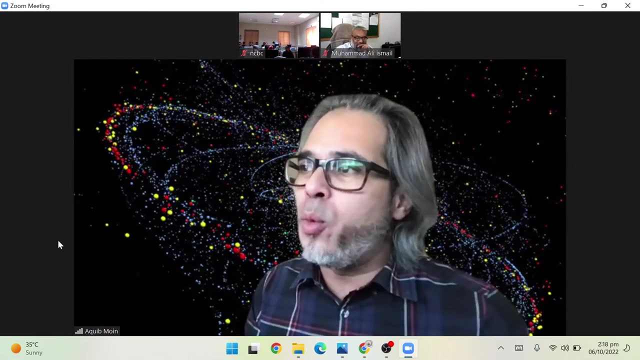 World Space Week activities. So, as you know that this year's theme for World Space cooked week is, uh, space, sustainability. so I thought that why don't I tell you a little bit about this whole sustainability issue and what kind of opportunities are associated with? 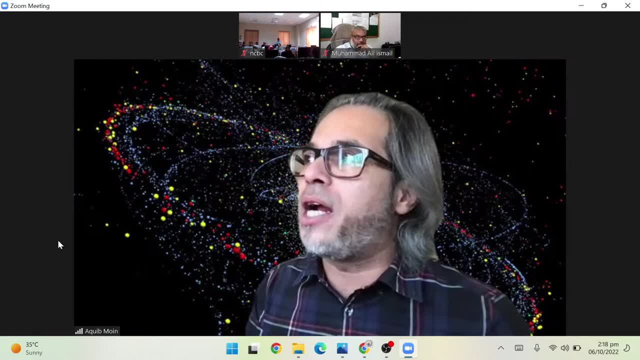 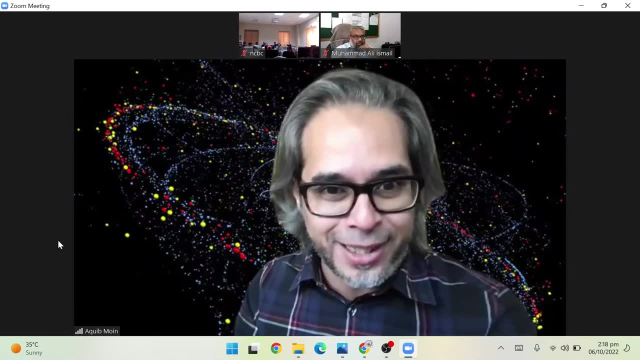 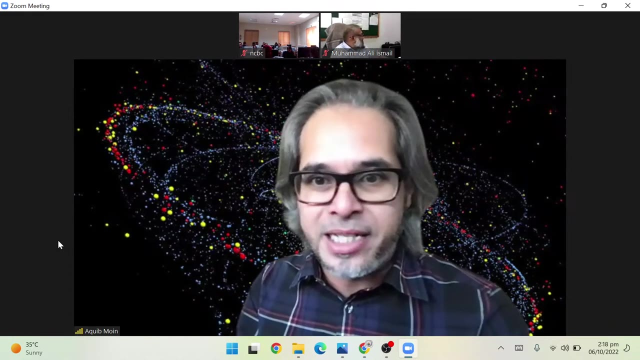 it Because you know, we hear sometimes. you know, We hear we will keep Urdu-English mix. okay, Because there is a Pakistani audience and we are originally from Pakistan, so we will keep a mix. So no hesitation in answering questions. 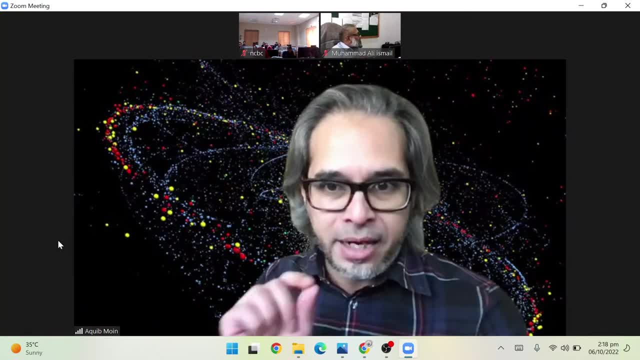 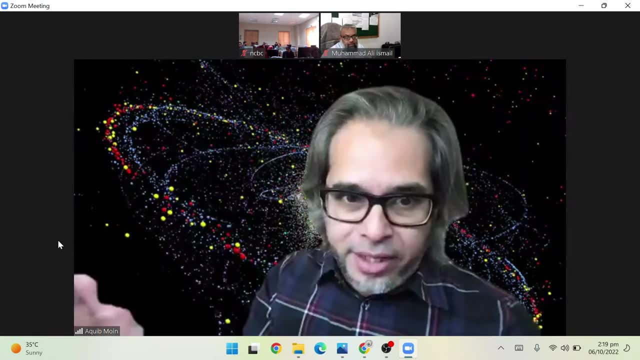 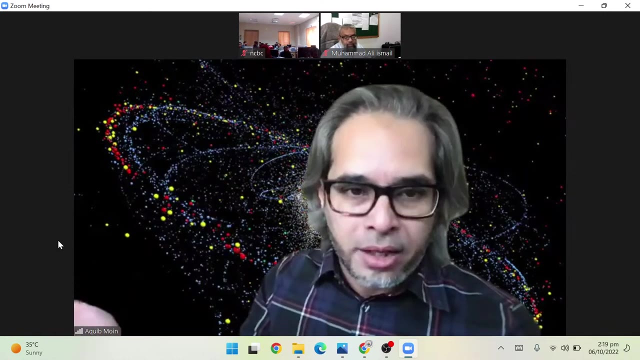 Whatever comes to your mind. you have to stop me and ask: Don't wait till the end, okay. So what I was saying is that when we talk about space industry or the space domain, they are: you know very large words and keywords and you know jargon that we use. 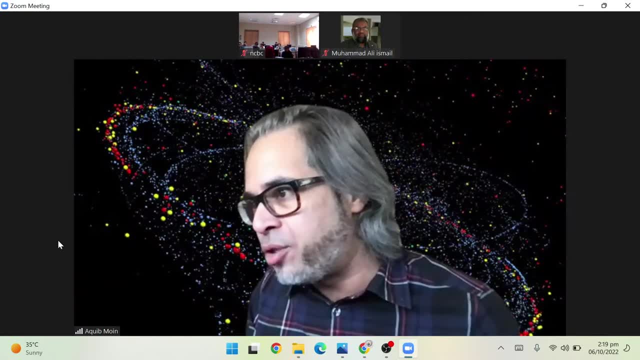 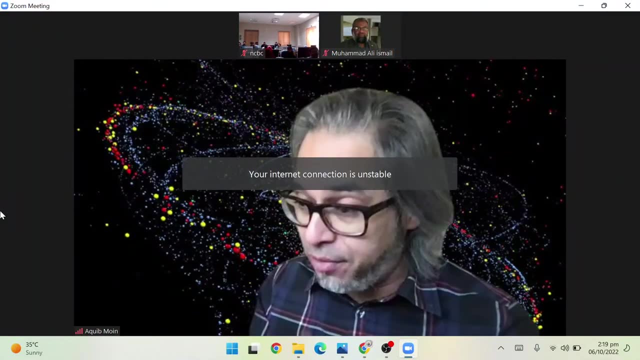 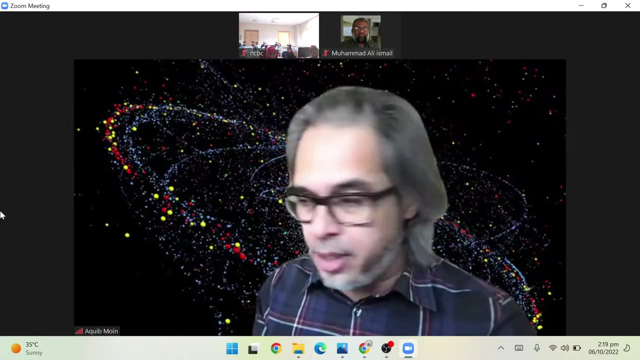 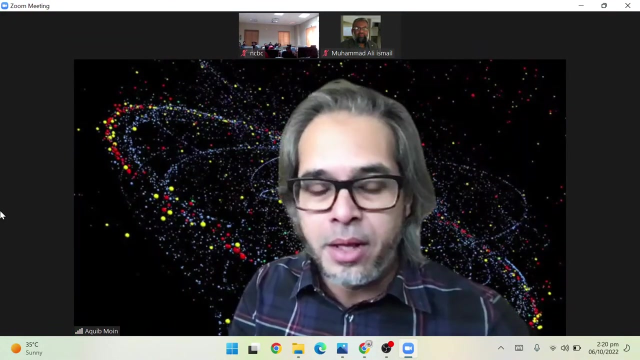 But again, what we sometimes do not grasp fully that what does it involve? because I myself am developing a space sustainability infrastructure here, which is us to do. right, Let me share my screen and then we will move on from there. So you know. 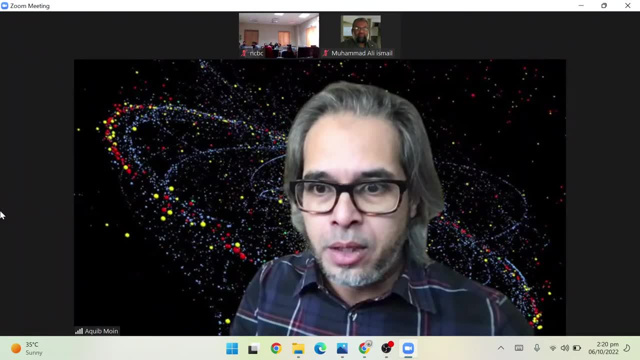 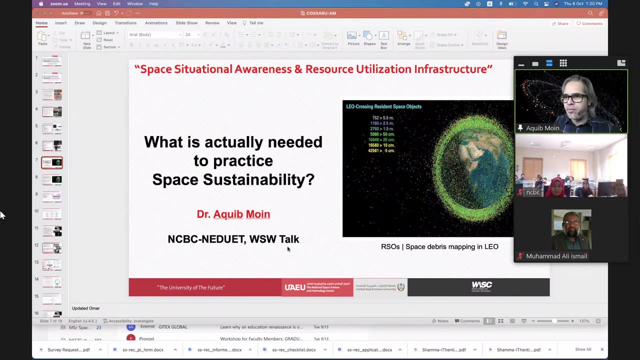 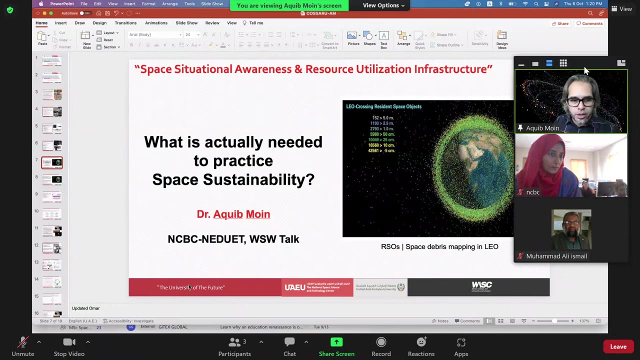 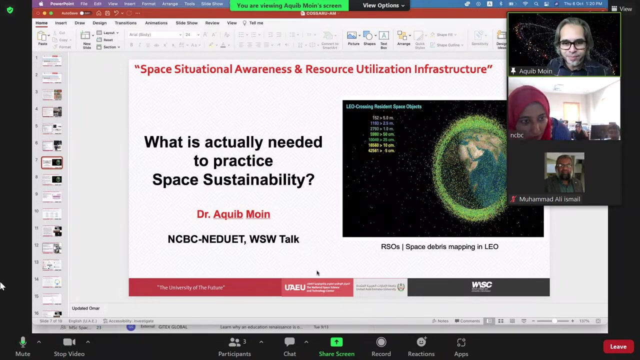 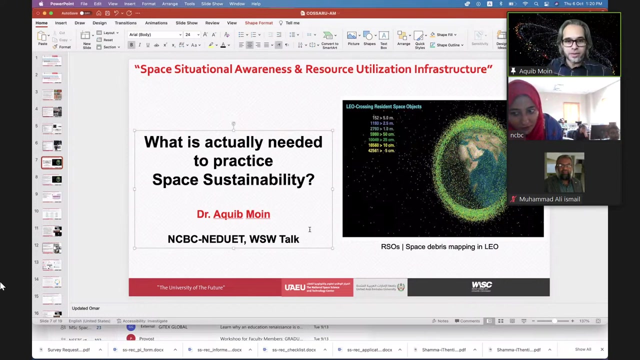 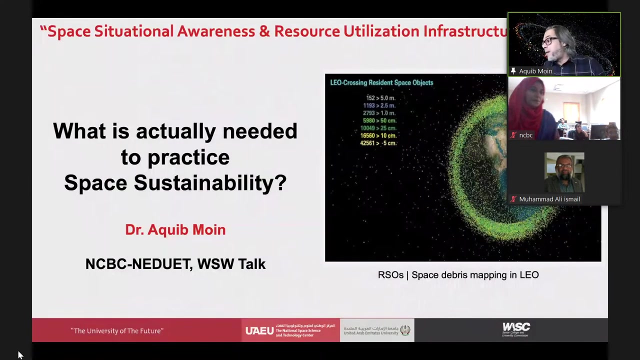 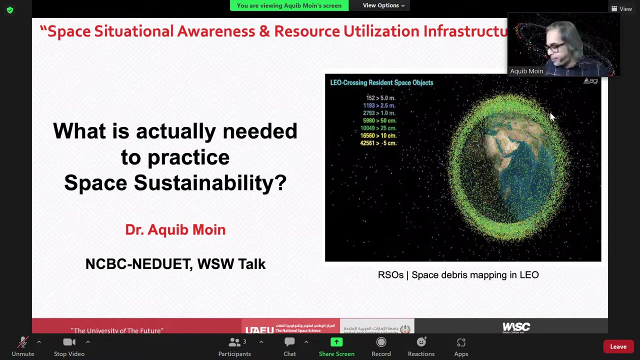 let me share my screen and then we will move on from there. All right, that sounds good, Very good. So we have a diverse audience with us today. So I think whenever I talk to a diverse audience, I try to keep things at a generic level, right? 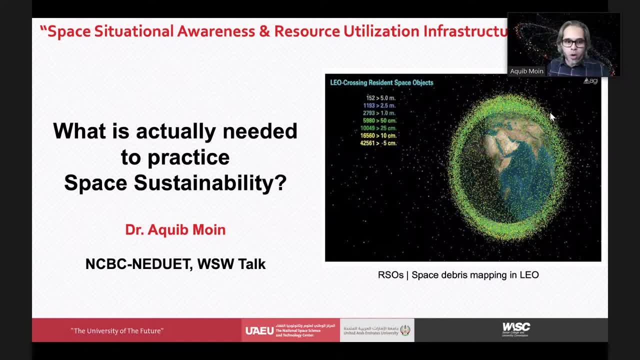 So I don't delve too much into details, because I want to address people who can, you know, equally grasp the basic ideas. I would say So even today: we will stay at the surface level, We won't go into too much of detail. 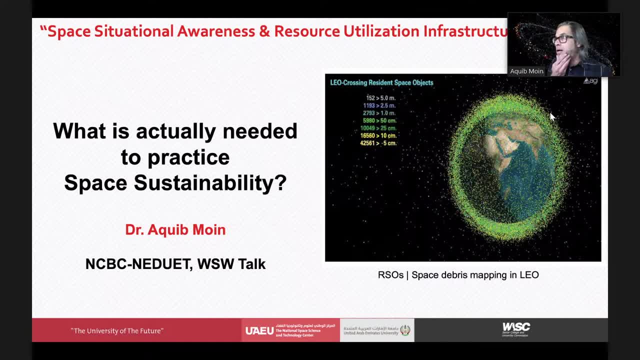 First thing that I would like to tell you about the space domain that it is extremely, extremely, extremely vast. When you use the word space science, space technology or space domain, it actually involves a very large number of overlapping disciplines. There is not a single thing in it. 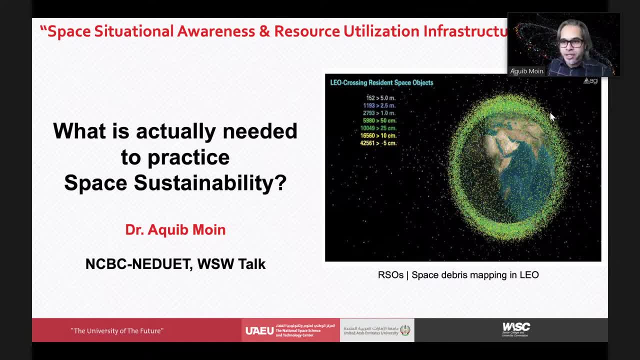 I think it absorbs all of the engineering disciplines, electrical, computer, mechanical engineering even, and all the other aerospace engineering, And also it absorbs physics, mathematics, chemistry and very heavy doses of, let's say, analytical geometry and so forth. 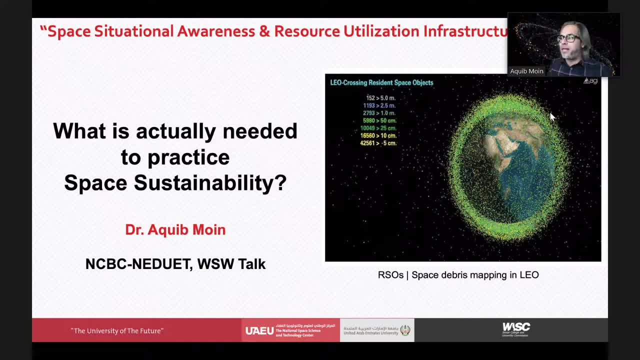 So first we have to understand about space science and space technology that it is not a single discipline or a single thing. What happens is that a lot of people focus on a single thing, but at the same time they are very much required to have a good understanding. 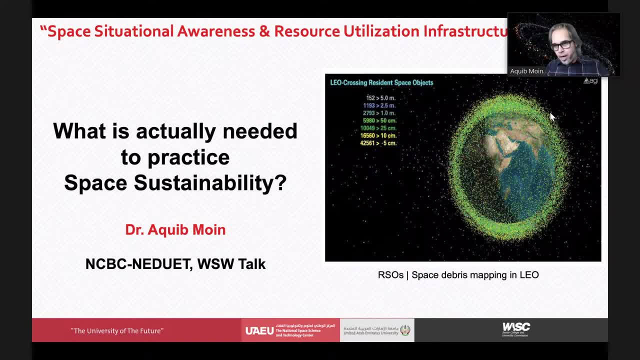 of various things that feed into the program. So I will also tell you that today, when we talk about space sustainability or when we talk about large-scale space projects, how different disciplines enter into it. Okay, So that is also important in terms of. 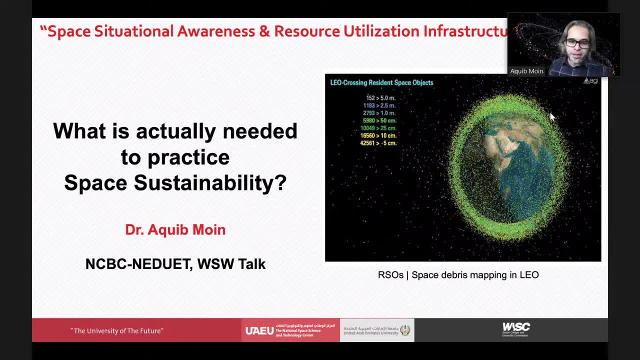 building up yourself for a career in the space sector. Okay, And regardless of what discipline you are, it doesn't matter. The space sector absorbs almost all kinds of disciplines. Right, Let's come to the point now. So I will not. 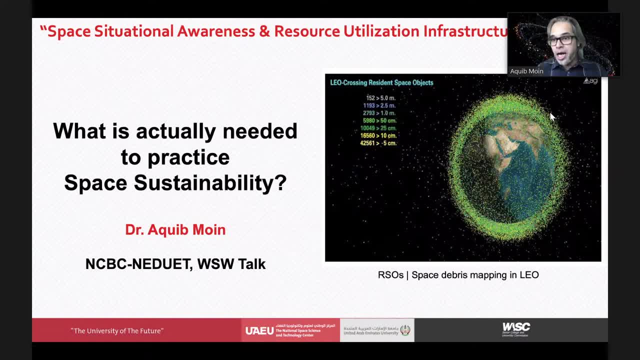 actually I will not take. what do we need to practice it? I will answer all three questions. The first question is: what is space sustainability? The second question is: why on earth is it needed? Why did you raise the question of space sustainability? 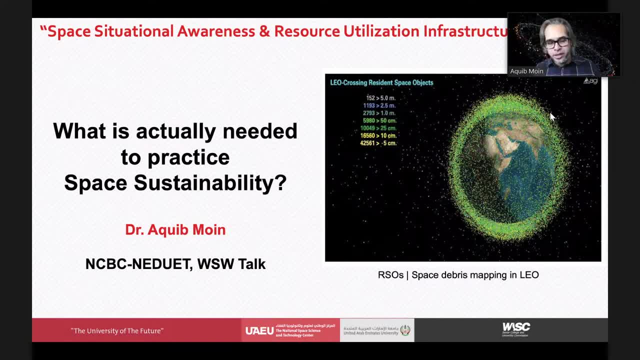 The third question is: how are we going to go towards the practicing of space sustainability? Okay, If you look at this image which is on my screen right now, it shows you earth surrounded by millions and millions of dots. Right, So let's start from this. 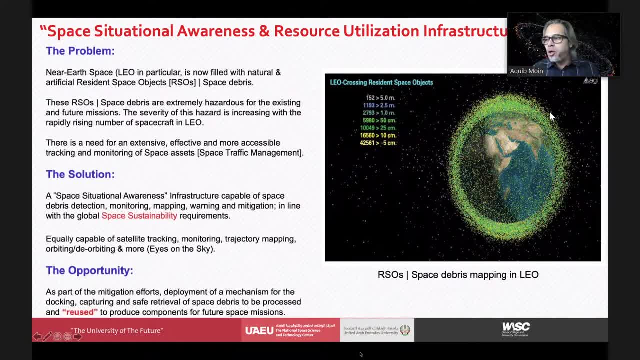 What is happening. So when you in your childhood or a few years ago, if you think about the space sector or if you see something about it, then in your mind, what would be the first word that comes to your mind? 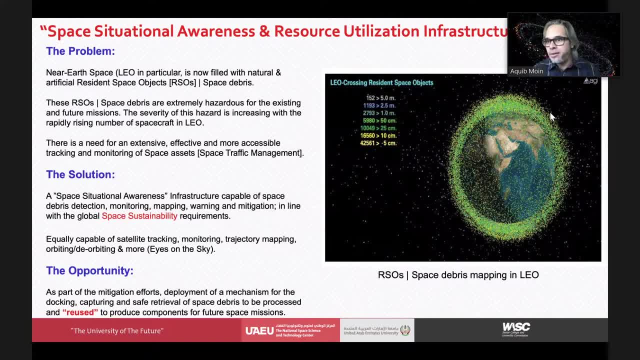 NASA, Right, NASA, which does a lot of things, and these are projects. they explore the universe. So until, let's say, about 20,, 25 years ago, there were only a few key players in the space industry. 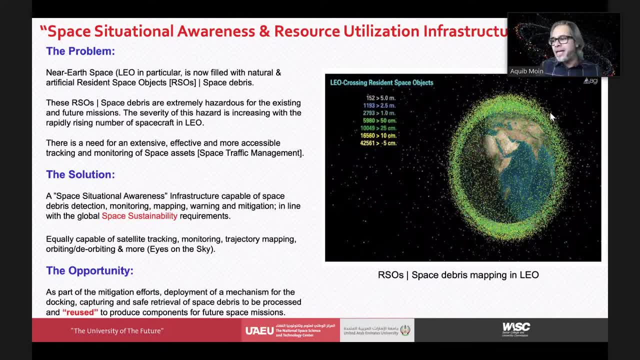 Right, There were only big names: NASA, ESA, JAXA, Japanese Space Agency- So they were the only few large-scale players in the space sector. And then there was a few large-scale spacecraft manufacturers, For example Boeing. 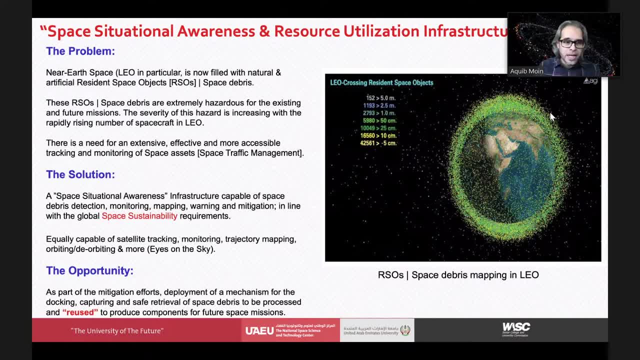 or Lockheed Martin or things like that. But in the last 10 to 15 years what happened is that the space sector has seen an enormous amount of boost Right Because of the emergence of the space private sector Right. A large number of private companies are being launched. 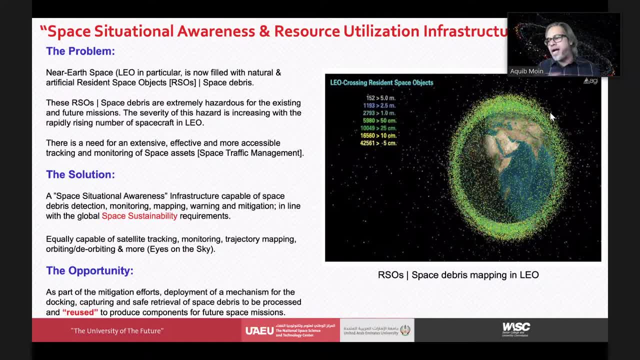 and they are involved in all kinds of space activities, such as CubeSat development or large satellite development, launching and operating and maintaining. So what happened because of that? What happened is that you know that all these objects 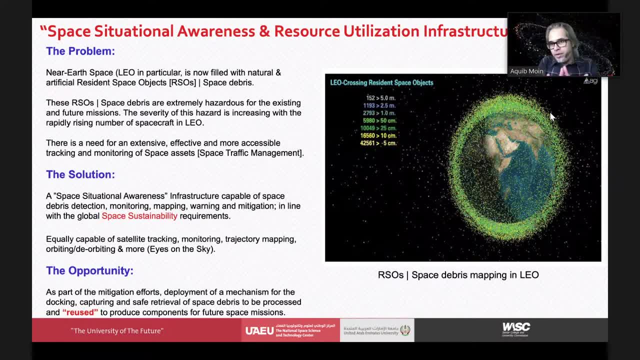 they orbit around the Earth, right? Whatever satellite you talk about, whether it is a communication satellite, or whether it is a low Earth orbit or Earth observation satellite, they all orbit around the Earth at different altitudes. Okay, So each satellite is orbiting the Earth at a certain altitude. 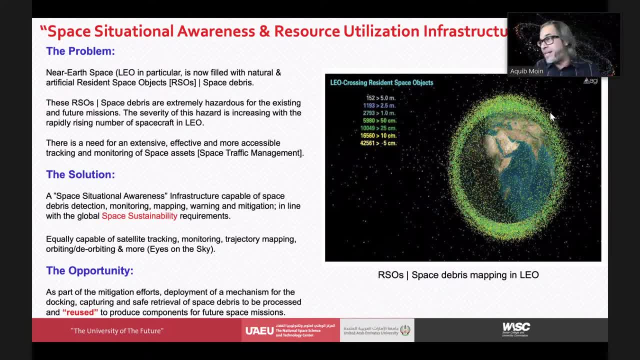 So what happened with the emergence and the boost of the space sector is that the near Earth space, right The orbits that are very close to the Earth, that space started to become really, really congested, So there is a problem of overpopulation in space. 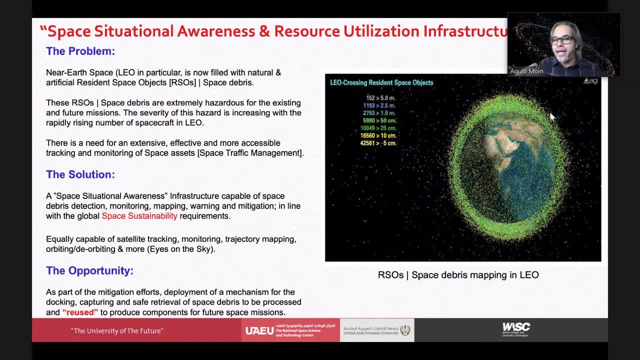 It is growing day by day. right, We are filling up space with too many objects, now right. But then the flip side of it is that we are launching too many satellites and spacecraft and all of that, but whatever dies in space. 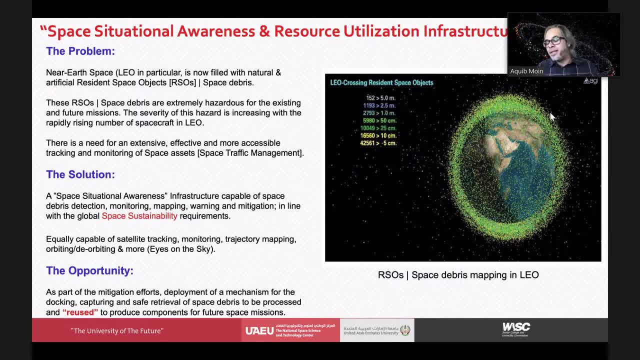 whatever spacecraft becomes dysfunctional or it ends its life, it is not brought back right. So in space, understand that space garbage is increasing a lot. There are dead satellites, there are pieces of rockets, there are, there are broken pieces of. 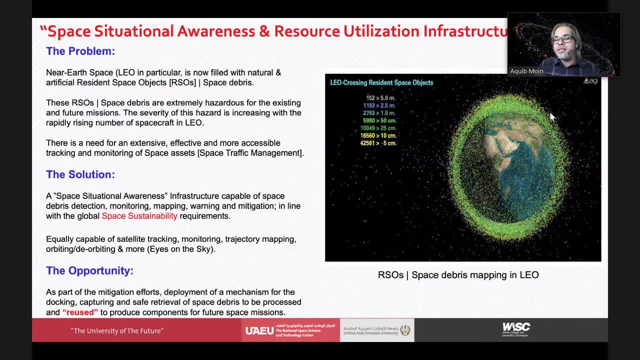 you know, damaged satellites. So what is? we don't care about it that much because you know space is not in our everyday experience. right Like here on the roads, someone starts a lot of garbage or 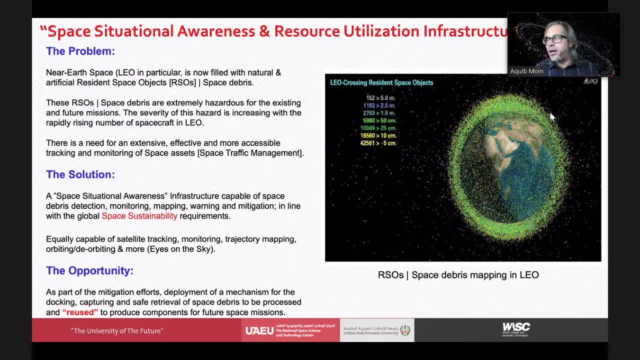 if there are too many cars and there are too many buildings, at some point you have to remove some stuff to deploy new infrastructure. Right, If you, for example, want to build a new building in some area and that area is already very congested. 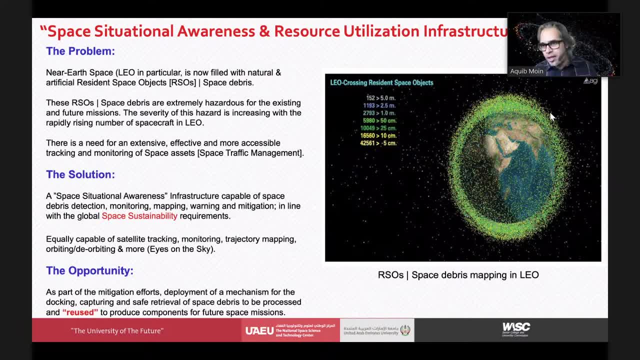 then what do people do? People first demolish an old building and build a new one instead. So what you do is that you keep on developing and deploying infrastructure, but you need to make sure that there is a cycle of 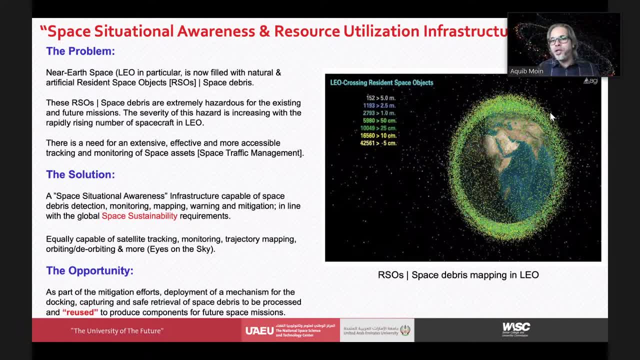 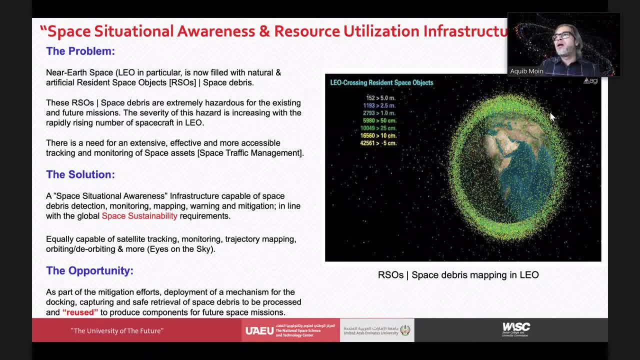 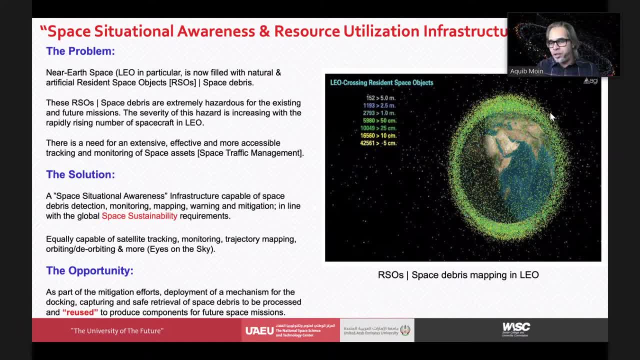 because it will either be hit by something which is already there or it would de-orbit due to a strike or something. So this whole situation is the primary concern when you talk about space sustainability. Space sector is growing, So we need to move forward with space technology development in a sustainable way. 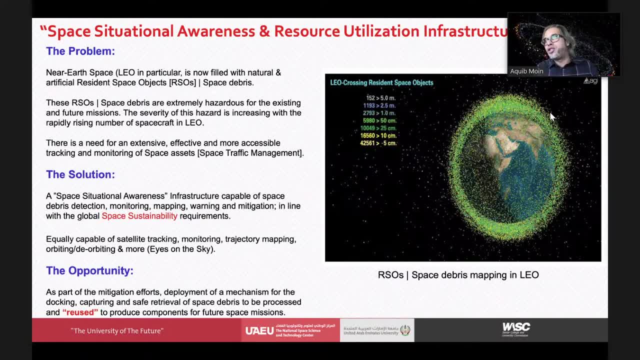 which means that it should progress in a way that it could continue without any blockage or without any problem, And for that, what is needed is that the space traffic right. First there is ground traffic, okay, But now there's. 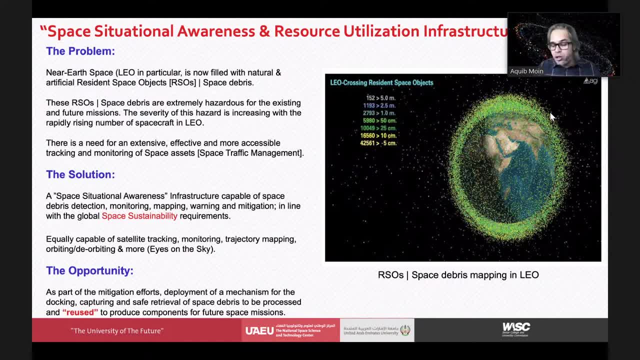 The number of spacecraft is too much in space that we also have an issue of space traffic. So the point is that space traffic needs to be managed properly, right, And we need to make sure that the entry and exit of spacecrafts is actually controlled and monitored. 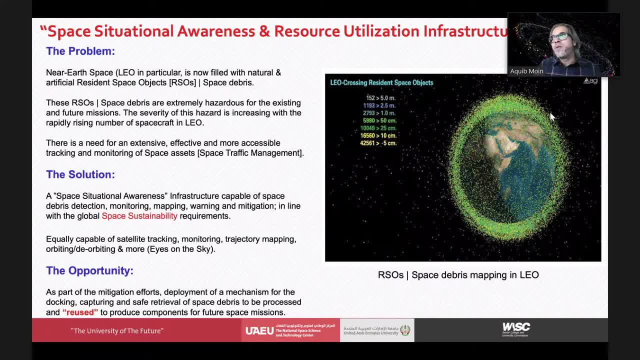 And we need to make sure that all of that garbage, those inactive satellites and all of that- you know, all of those pieces and the leftover from the other missions- is actually removed, right? So this whole idea of continuing to explore space in a sustainable way. 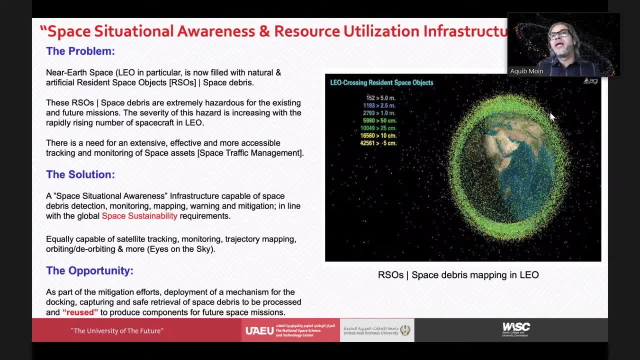 that it does not come to an end at some point because of our population. that is the narrative of of space sustainability, right? So now you can think that it is connected to a lot of things. Now, one thing we have done is: what do we mean by space sustainability, right? 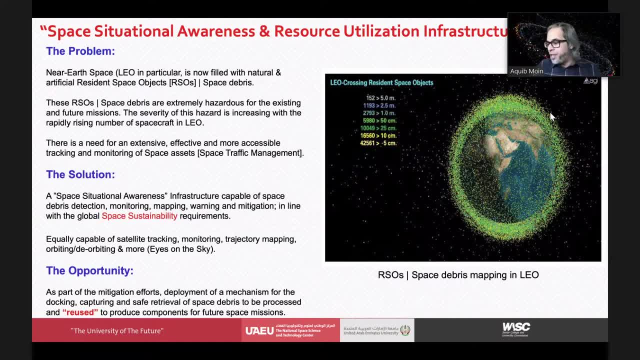 We are populating the near-Earth orbit and we need to find a way to launch and launch spacecraft in a- you know, in a well-managed way, and at the same time, remove the stuff that is not needed So that the exploration can go without any kind of discontinuation. 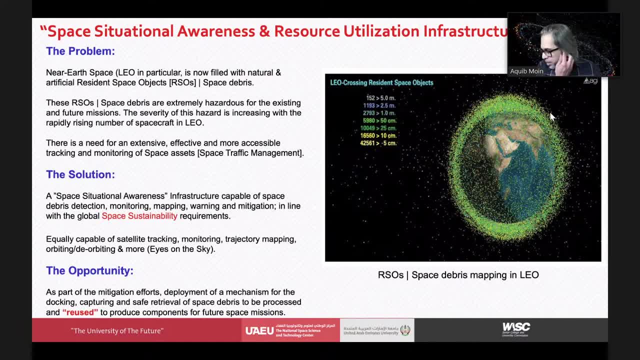 So now we discuss the second point, that what is needed to do this? Now, if we want to do this, how do we want to do it right? So the way the space environment is now being filled with a large number of spacecraft. 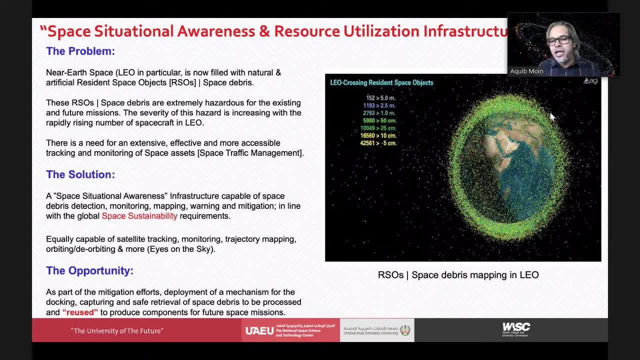 right. So you guys must be aware of the name: Elon Musk, right from SpaceX. So Elon is actually aiming to launch roughly 12,000 satellites. right, Jeff Bezos from Amazon. he actually owns a space company now which is called Blue Origin. 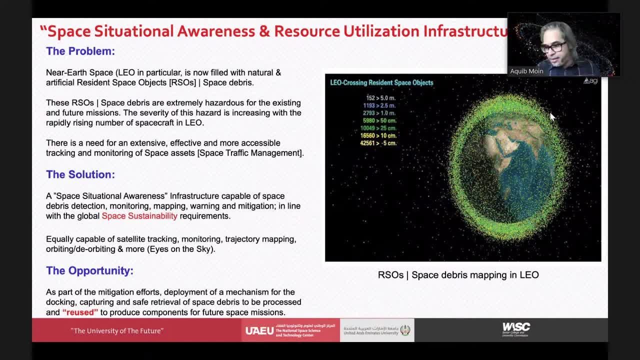 So he's trying to launch a large number of satellites and there's another project called OneWeb and so forth. So he's trying to launch a large number of satellites and there's another project called OneWeb, and so forth. So the point is that over the next few years a very large number of spacecraft is going to be deployed in space. 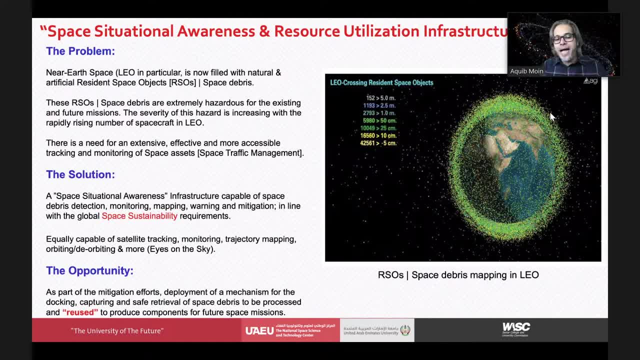 So what do we need to do? What is actually needed for space sustainability? So the first thing that we need for space sustainability is that we need to have some kind of process and methodology and some kind of an infrastructure that can actually track all these objects from the ground. 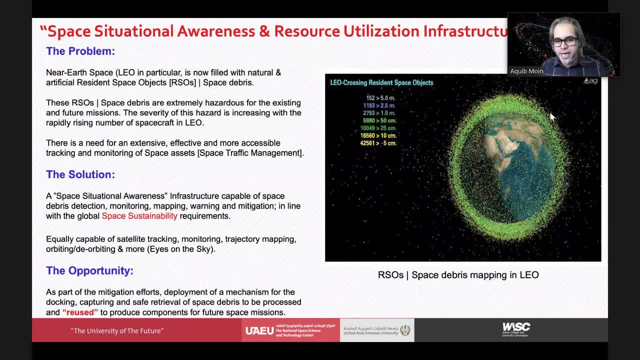 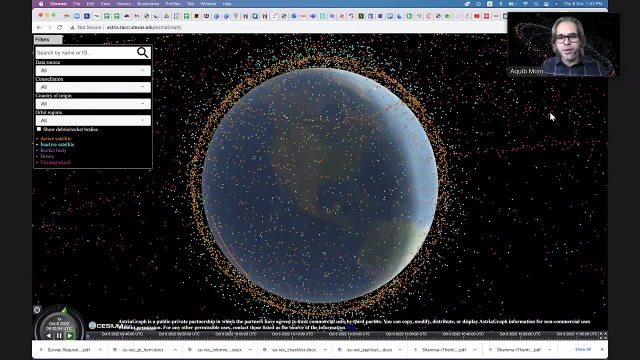 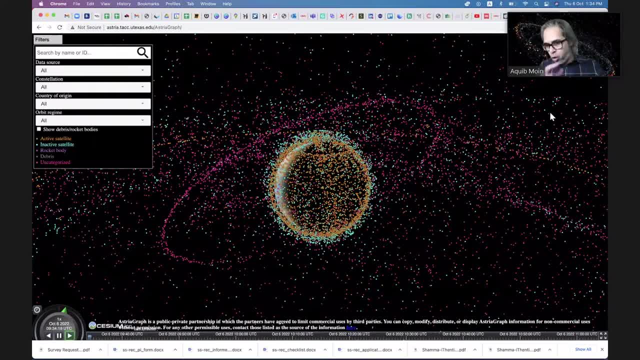 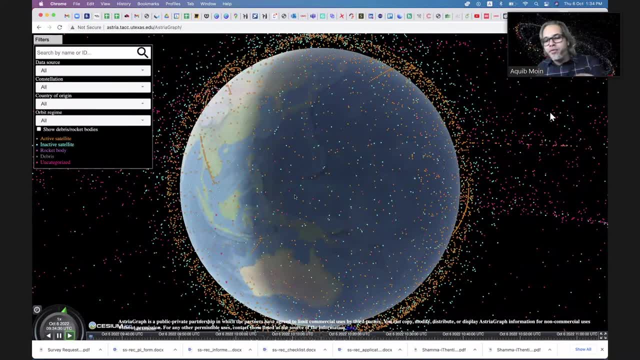 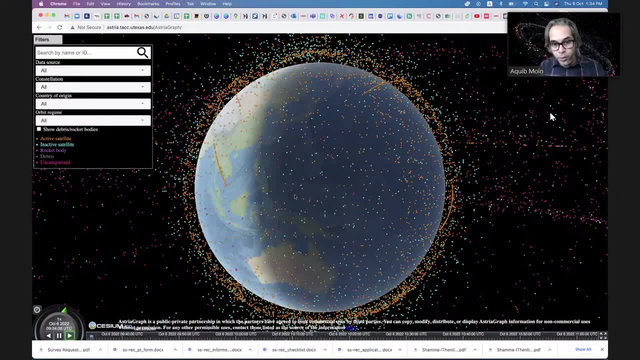 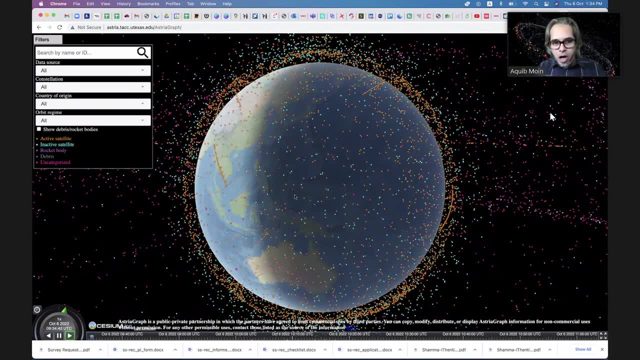 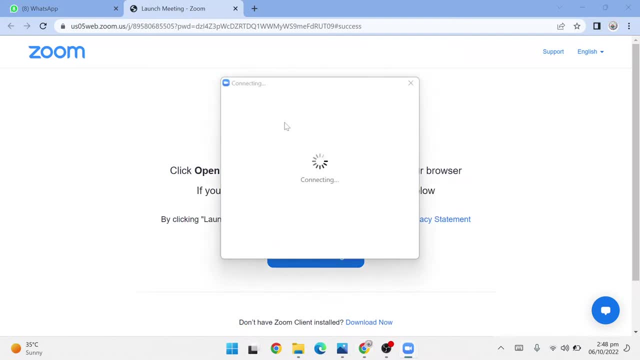 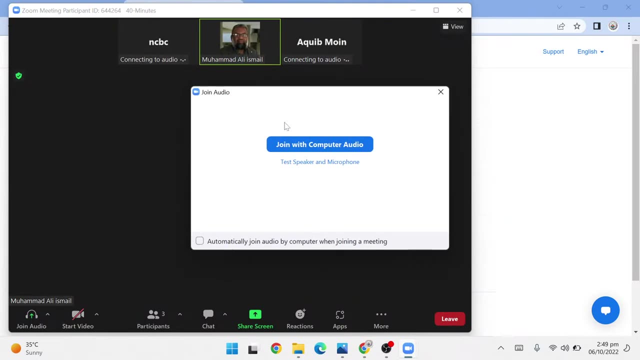 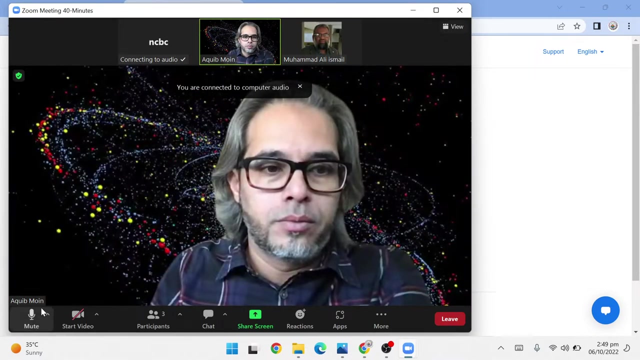 What we do is that when we launch a satellite into space, you know rockets are usually multistage right. What we do is that when we launch a satellite into space, you know rockets are usually multistage right. Hello. 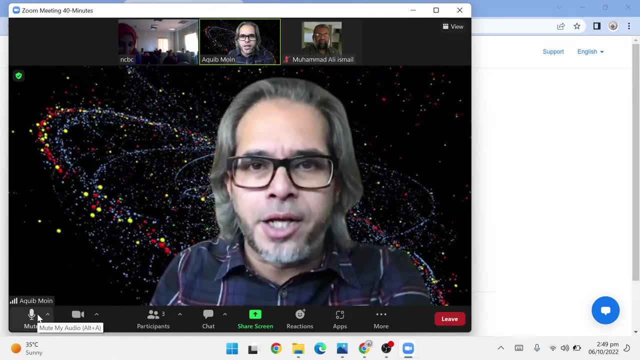 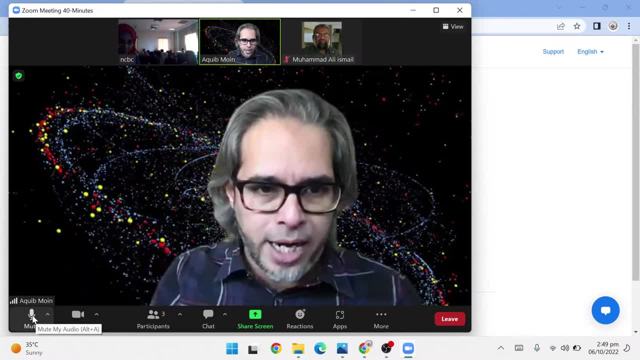 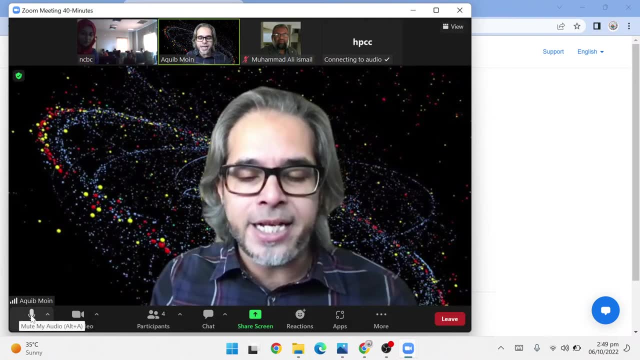 Oh, I think the session ended for some reason. I can you guys hear me now my presentation in a few minutes, and then i would like to uh talk a little bit more with the students and would prefer that, uh, we engage in a conversation, not just one-way uh speech, or 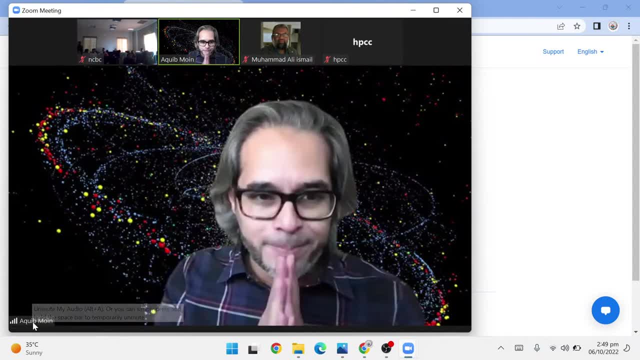 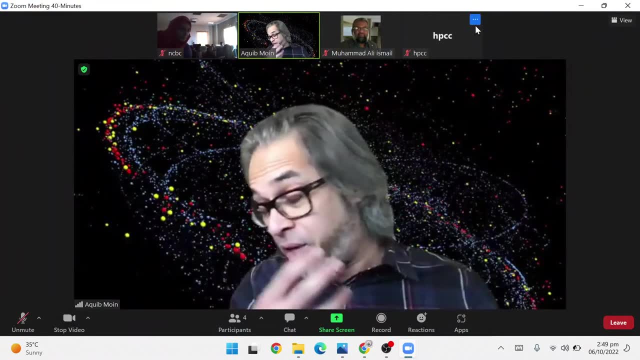 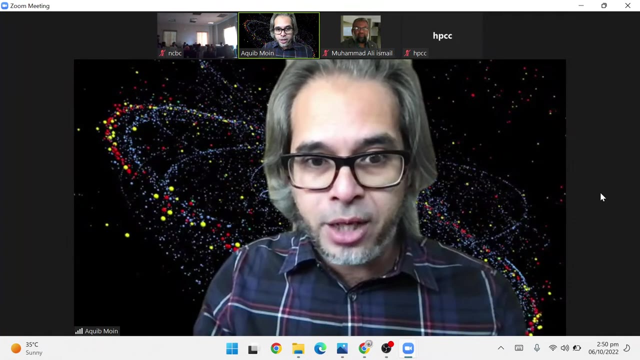 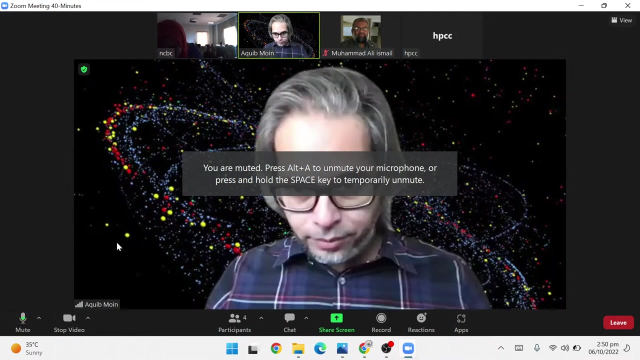 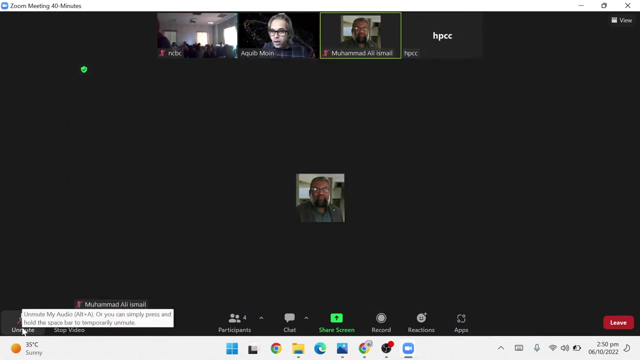 anything anyway, oh yes, uh, i was trying to tell you about the connectivity between different disciplines, right, uh, again, let me share my screen again. let's go, uh, here up so that i can share my screen. yes, okay, thank you, sir. thank you so much, so now i can share my screen again with you guys. 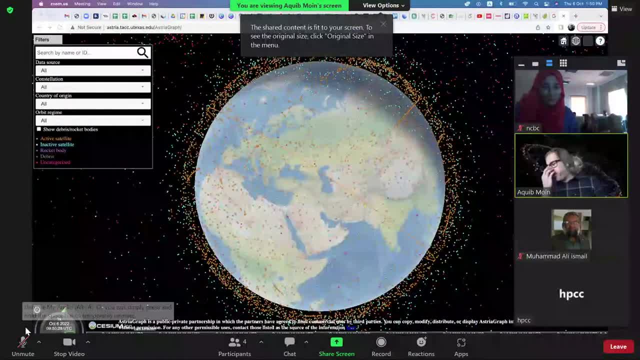 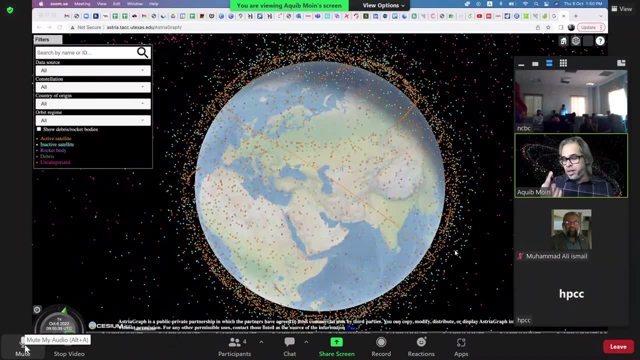 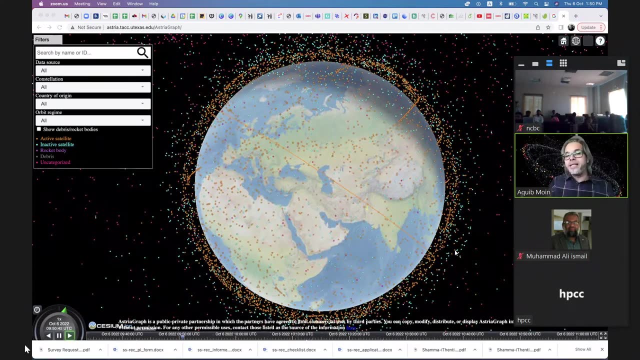 um, okay, so i think what i was saying is i i gave you sort of like an overview of what space sustainability is. number one, number two: what do we need to do when it comes to sustainable practices? and number three: what is that kind of- uh, what is involved in getting? 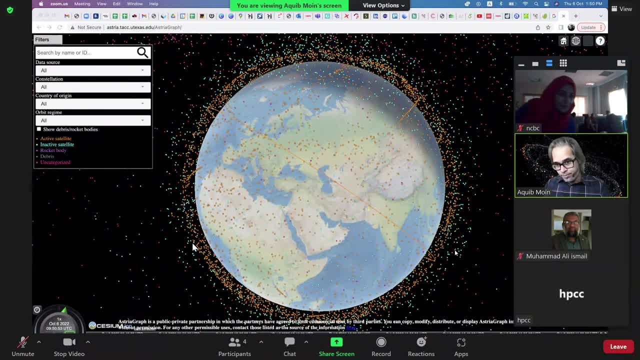 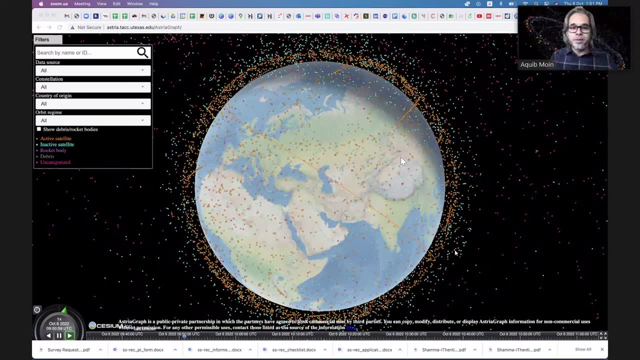 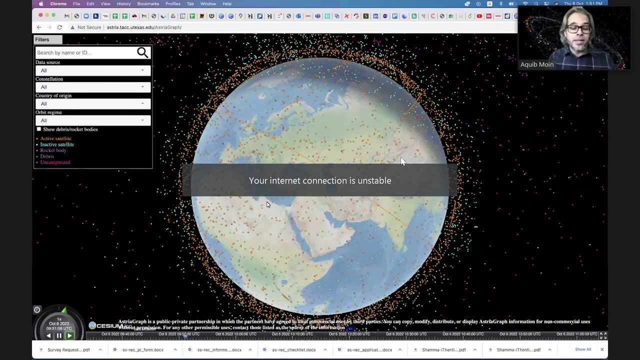 cover the question that why do we need to do that? right? so i hope most of you are clear, uh, that you know it. if you are, if you want to engage in something like this, then um it it. there are far too many disciplines that go into this activity. 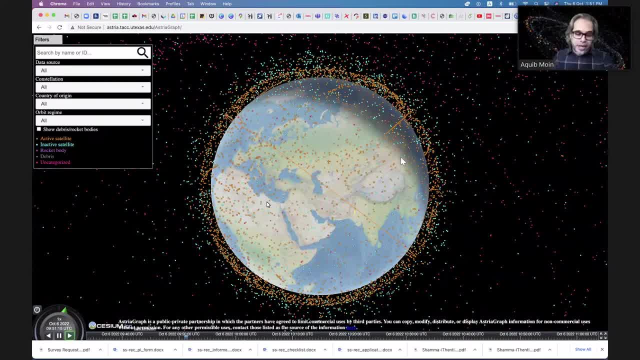 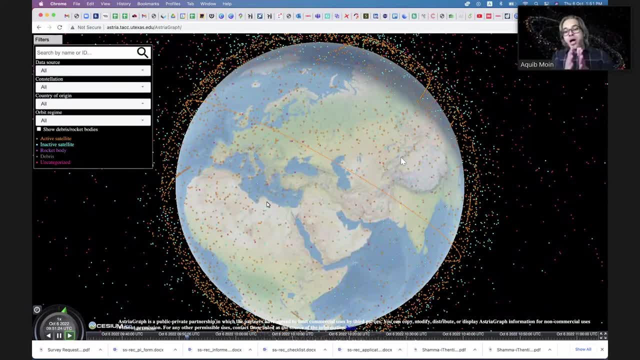 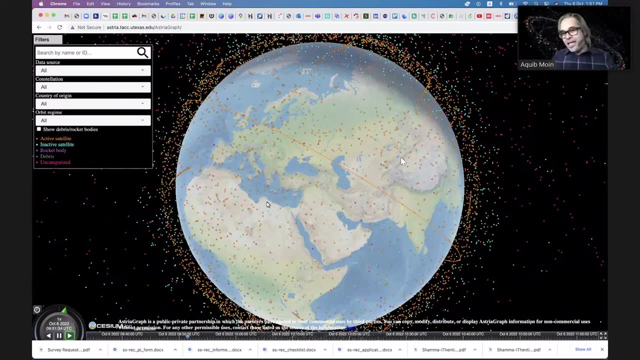 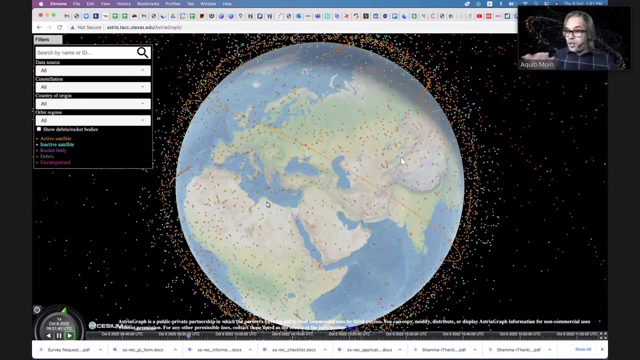 right. so it's not just so what i was trying to tell you- and i i always try to uh convince, uh, especially pakistani students on this- that go beyond your disciplines. now the world is not working with specific disciplines anymore. right, you can have your specific discipline, but then the if you want to get into advanced research and science, you need to go. 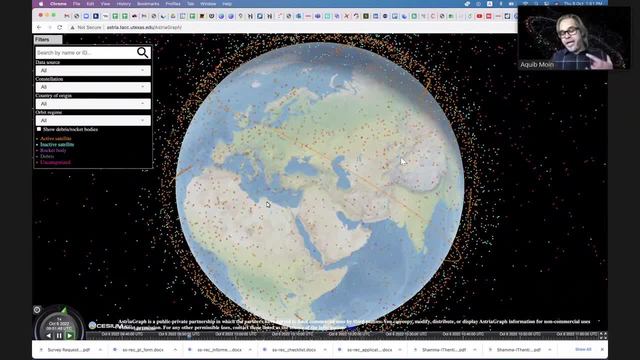 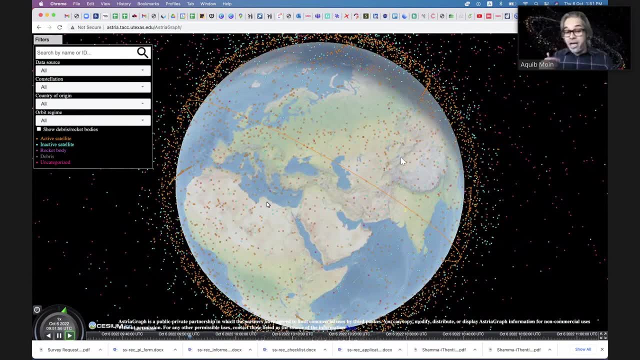 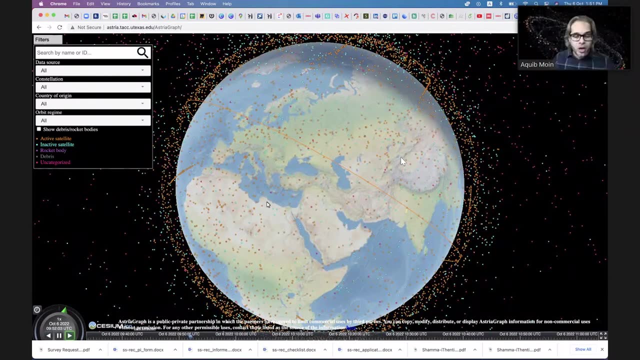 beyond that, you need to have expertise in- let's say a few more things- software programming, uh and uh especially. or, if you want to get into space sciences or space technology, uh, it's very useful to understand orbital mechanics, or celestial mechanics and the motion of satellite orbits. 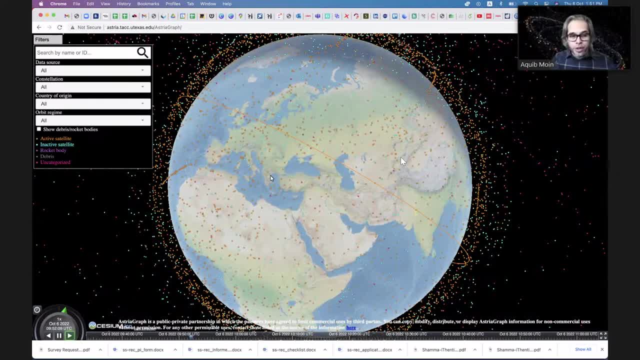 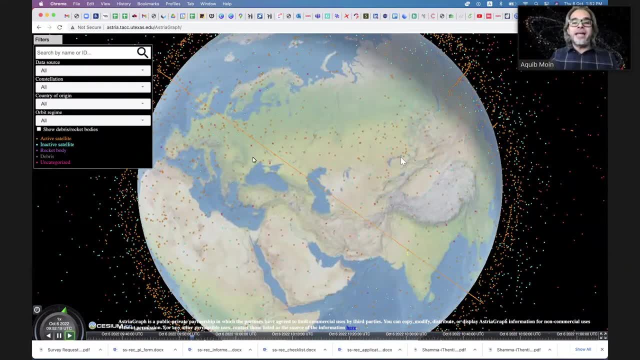 satellite dynamics and the satellite, uh, attitude control and so forth. anyway, that's that. that was just a side pep talk, so, um, but again, you know, it's a very highly multi-disciplinary activity in which we start from a very high level of multidisciplinary activity in which we start from. 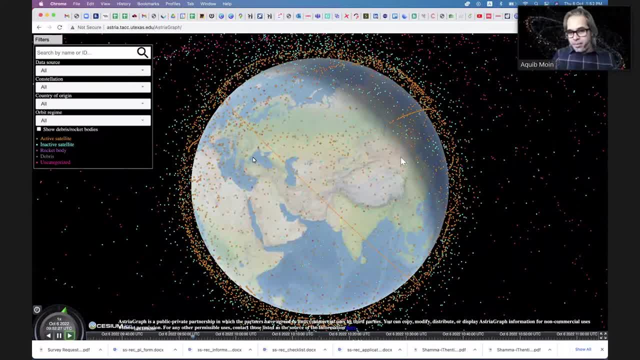 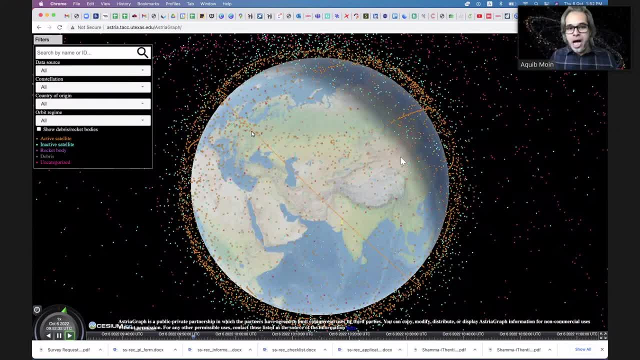 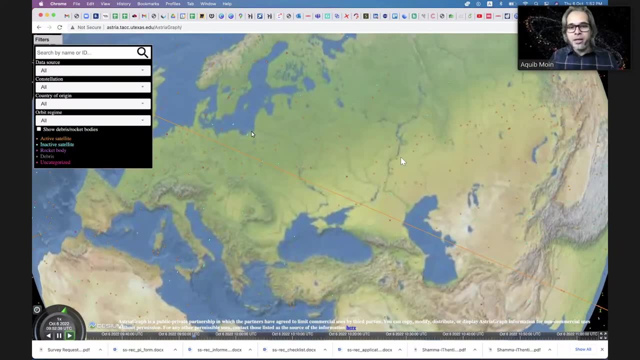 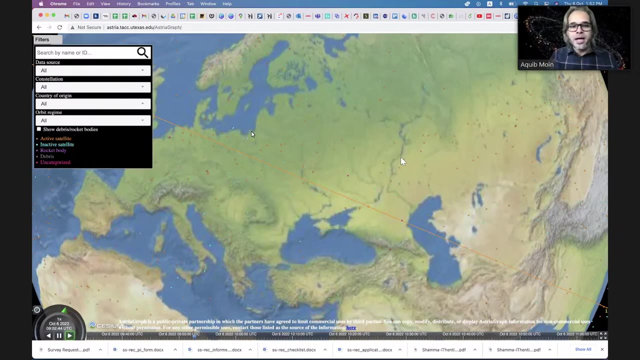 building an understanding of the satellite motion and its dynamics, and then we try to learn from its motion, and then we try to see that how exactly are they uh moving above the earth right? and then we process all of that data to ensure that uh, the space exploration and deployment. because you know one thing you might ask, i think: 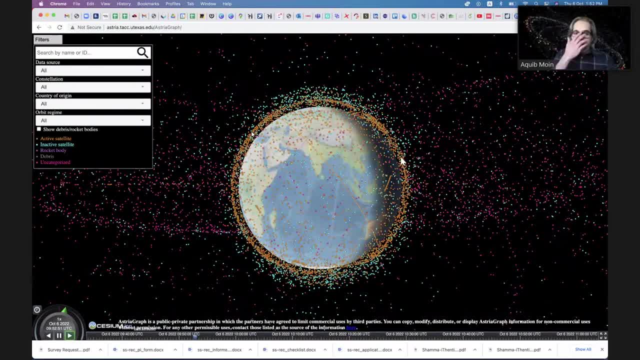 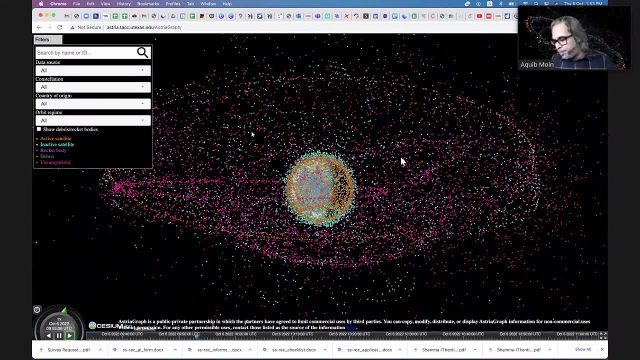 my last few comments will be that: uh, so once we have this data one, once we have analyzed all the dynamical parameters, and once we have established that how, we will make sure that the satellites will not strike with each other and there is no overpopulation, based on all of this study, what we have is a careful and well-managed plan as how and where to 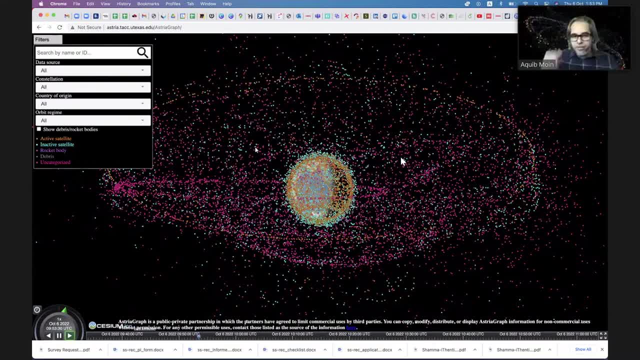 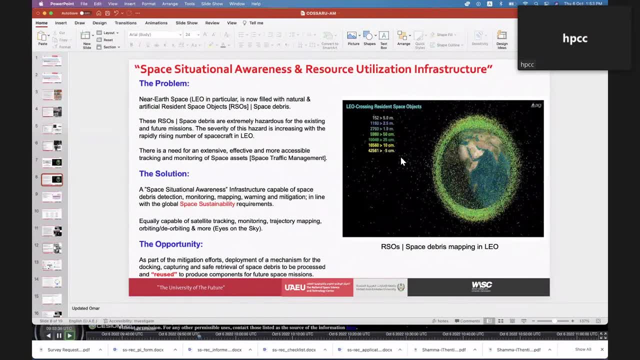 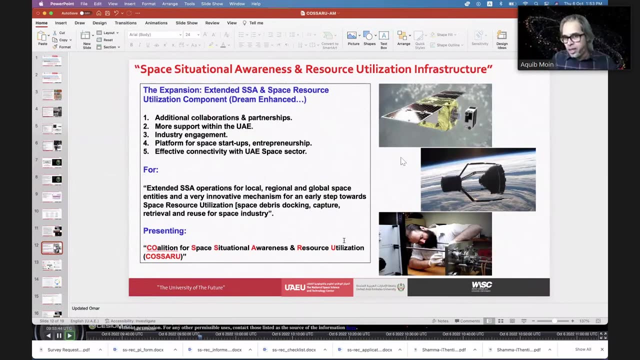 deploy a satellite and what kind of stuff we need to remove from there. so let me give you another example on this. so what we are also working on is the removal of unwanted material. so the funny thing is, we need to launch a satellite to remove a satellite from space. 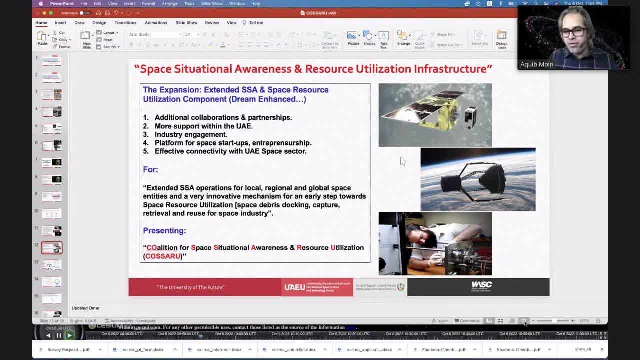 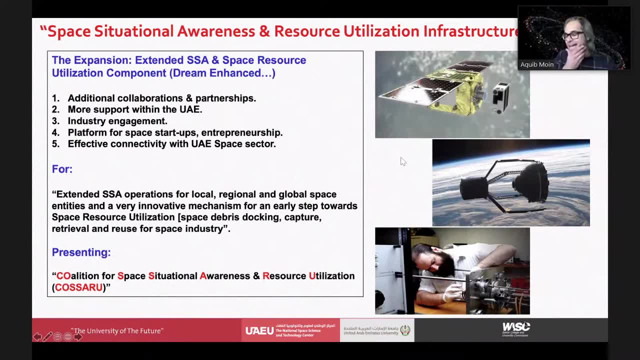 right, right. so also trying to achieve under the heading of sustainability is that we are going to uh launch satellites which are capable of capturing the unwanted stuff and bring it back. it might sound crazy, but we are working on this with different uh collaborators, so you can see. 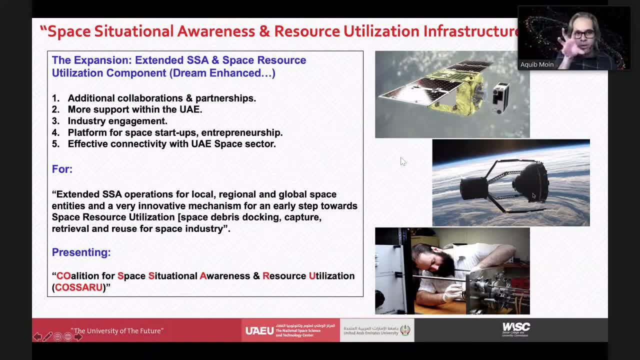 that one possibility could be that there is a claw- right, it's a Punjab- there's a claw which can grab this- uh, unwanted piece and it will bring it back to Earth and then we can recycle it, basically so, space recycling- as crazy as it might sound, that is something that we are working on. 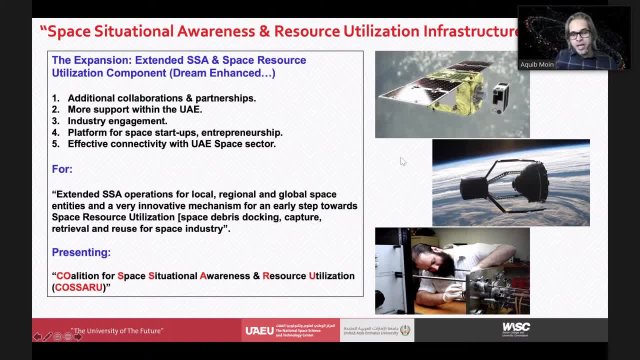 then the other technology that we are working on is which is called magnetic docking. you will have a space spacecraft which will have a very large and powerful magnet that will actually capture all of the metallic debris right. when I talk about unwanted material, we usually call it space debris. 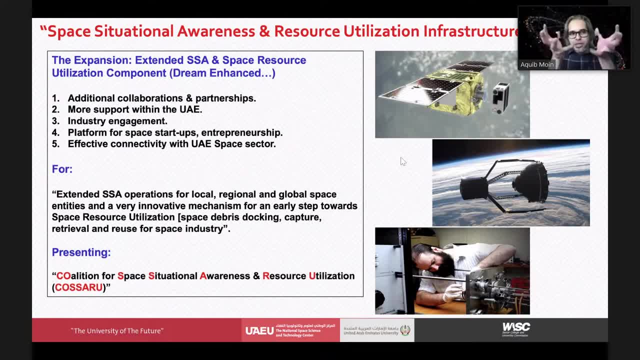 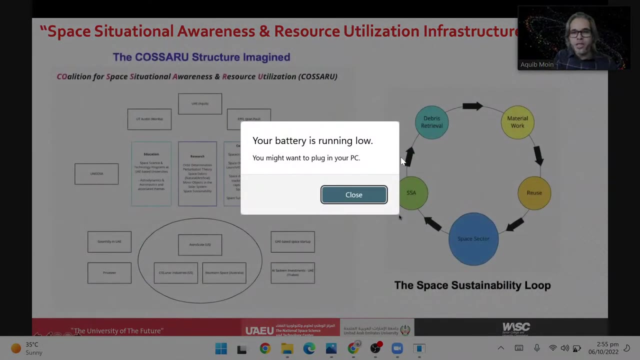 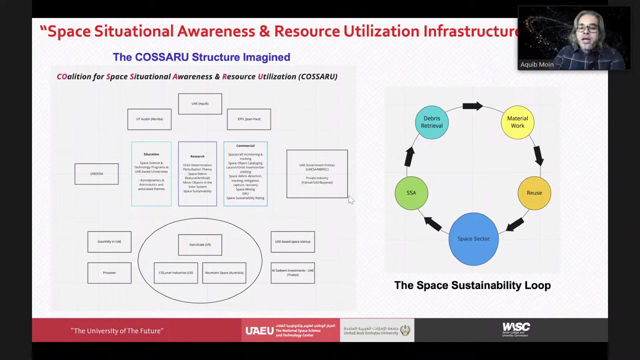 right. so these uh magnets: they will capture, uh, the metallic degrees and they can actually bring, bring them back through re-entry and we can actually recycle that. so that's so. that's an amazing thing about this. uh, so once we recycle all of that, uh, so this is what I wanted to end with. so we have. so space sustainability Loop right, so we. 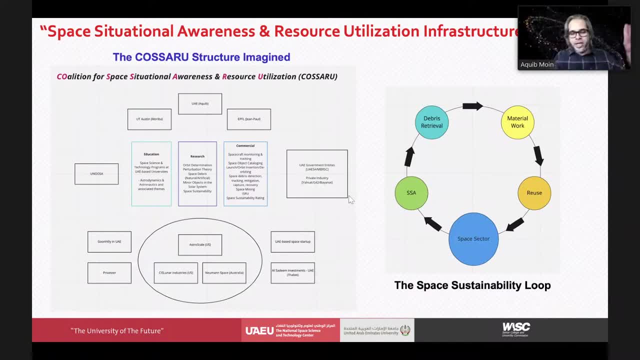 have the space sector. we are launching satellites, we are launching uh, spacecraft and missions and different purposes, so but what we need- and- and this is getting overpopulated- what we need to do- is we need to do space situation Awareness. we keep an eye on all of that. we manage the entire Network of satellites. 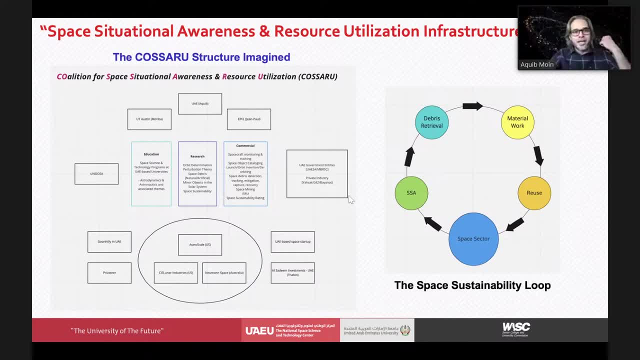 properly. we manage their motion, their entry, their exit properly, and then we found out what is the stuff that is not useful. we bring it back and then we re reuse it. so that is something that completes the whole space sustainability Loop, right. so so that's what we need and that meets the good. 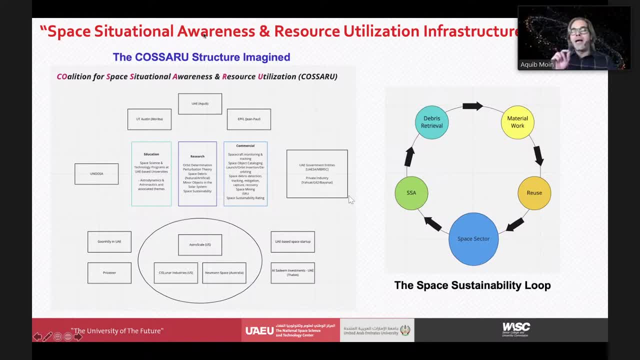 so you achieve space sustainability by making sure that your operations and exploration goes continuously, that new, new spacecrafts is are launched and the garbage is well managed, based on scientific study of the dynamics of all of the objects. right, so i think i have. i mean, we can have a very long conversation on this. um, i think i would. 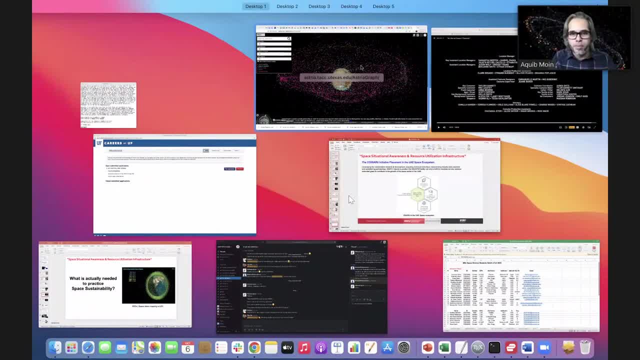 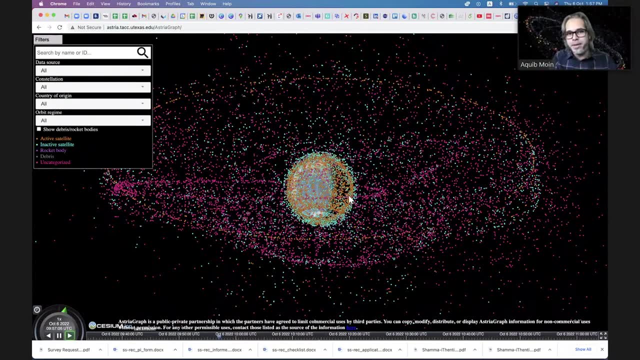 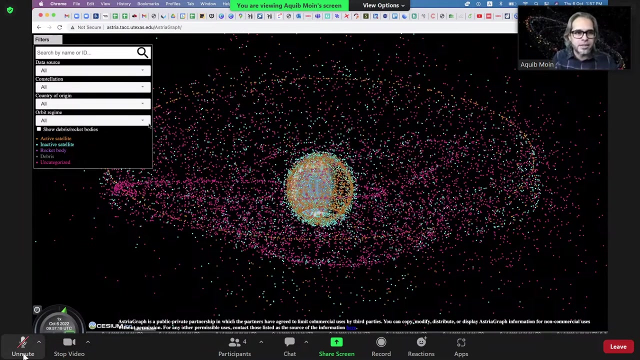 uh, stop here, right, and i will go back and i will stay on this, uh, uh, this simulation here, or maybe, you know, i can just get into a larger window or something. um right, so i think here that's where i would stop and i would welcome any questions and if you can turn on the lights at your end.